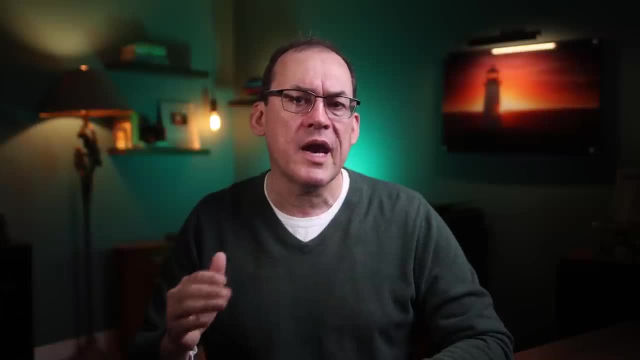 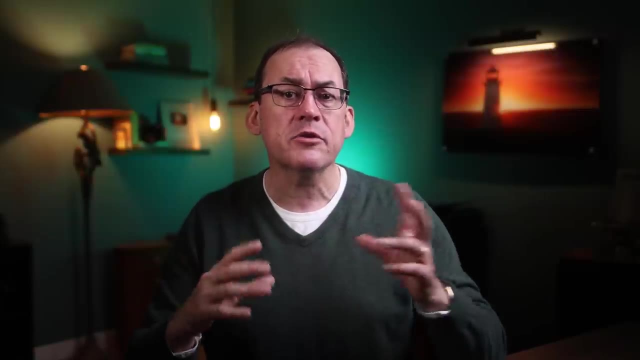 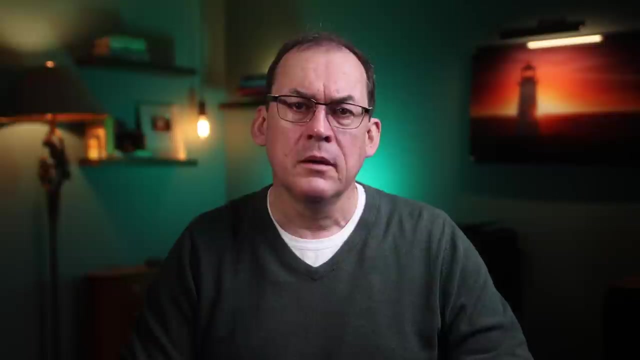 There is indeed a relationship between price and the features your camera and lenses will have. A larger budget will likely buy you more. The budget will allow you better build quality extra features and maybe discretionary attributes like weather sealing or two card slots, which are important for professional work, but less so. 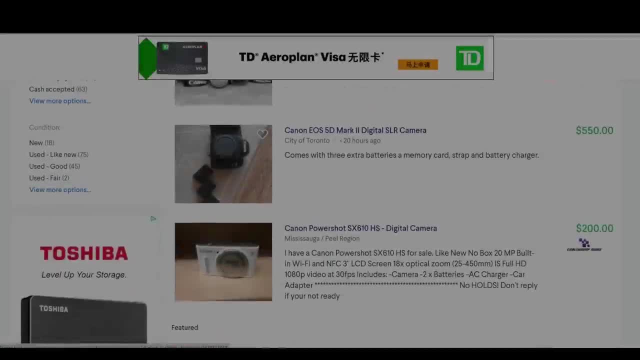 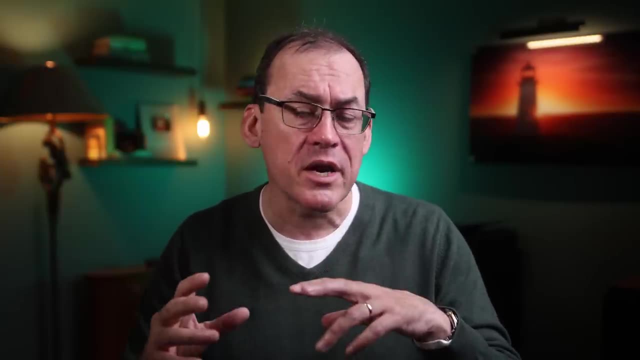 for the hobbyist. You can indeed make your budget go further by buying used. I've bought used gear before and there's nothing wrong with it. You can often get more features and better cameras using the discount that's inherent in used gear. When buying a used camera, ask how many shutter. 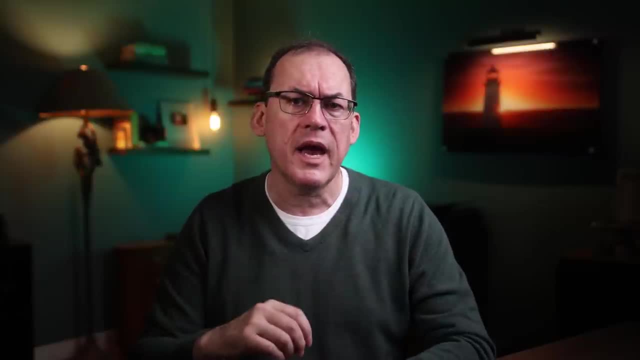 actuations it has. Some cameras track this or you can get apps that get this information from the camera. Shutter actuations are a common feature for camera manufacturers that will be more likely to be used. However, if you're looking to buy a used camera, you should be careful about the number of 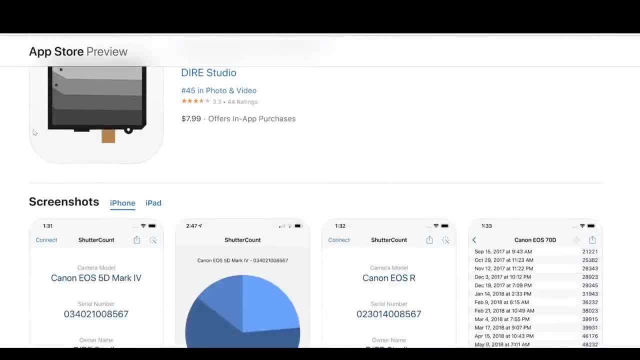 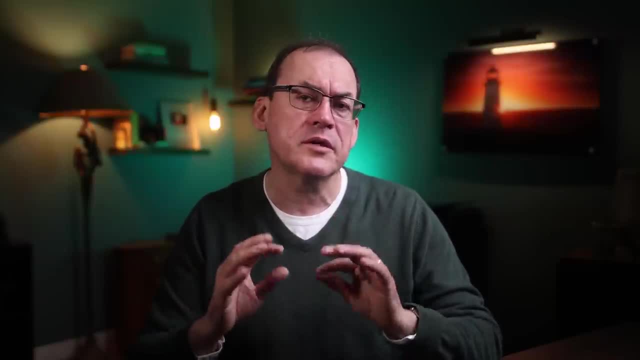 Cutters on high-end cameras can last 300 or 400,000 actuations or more, but in some beginner cameras 100,000 is a lot. If you get one with under 50,000 actuations, there's probably lots of life yet. 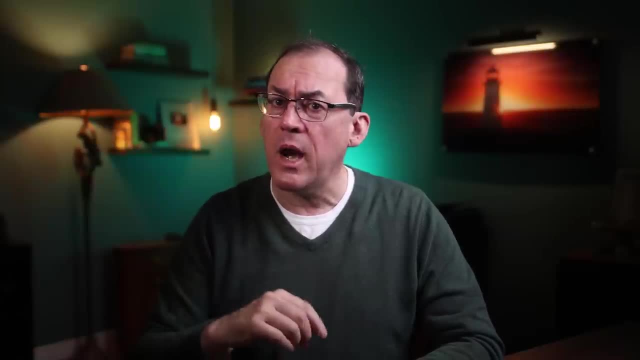 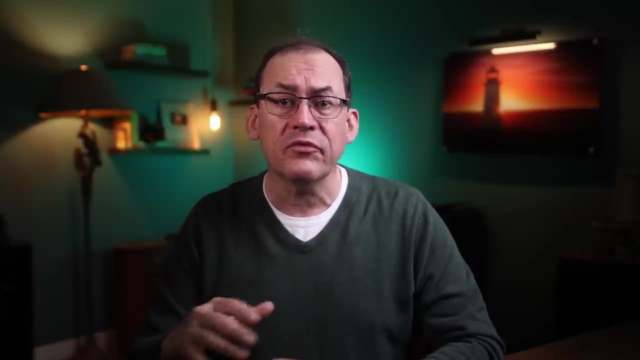 Also ask whether or not it's ever been dropped or serviced and why. The biggest consideration in used cameras is whether or not you can afford to repair it if it breaks down, While the odds of you using it for years are in your favor if you can't afford the cost. 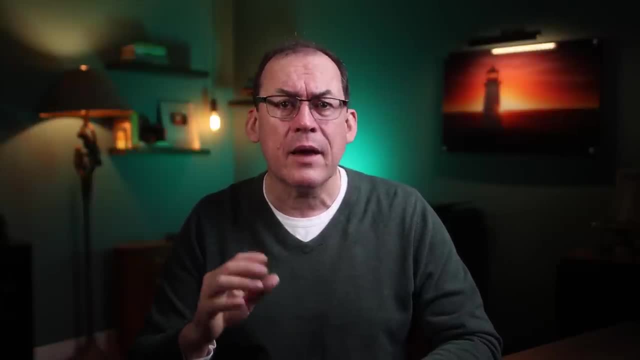 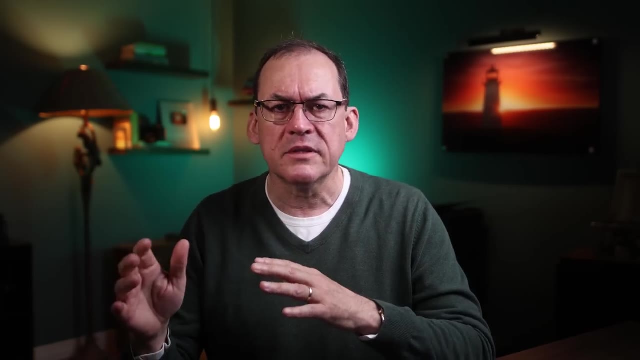 of a repair. if you need one, then it's best to buy less camera. but new Cameras these days are divided into two technology camps: DSLRs and mirrorless cameras. DSLRs have a mirror in front of the sensor that needs to get raised to take a photo. 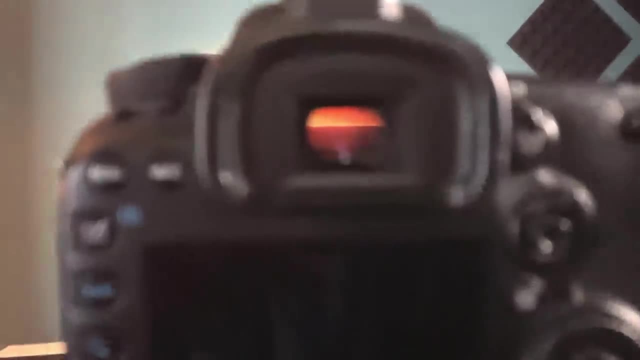 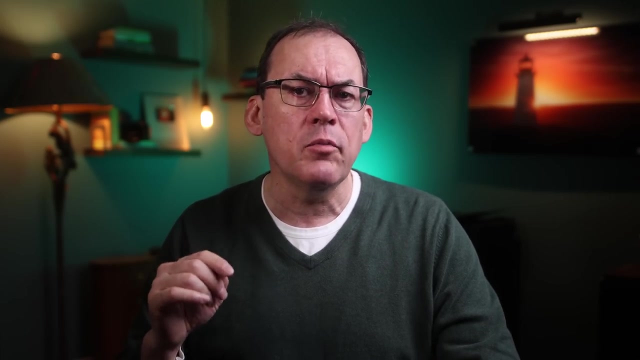 It also has an optical viewfinder, so you see what the lens sees as a live image in real time. As such, they're usually in a larger form factor. Mirrorless cameras, on the other hand, have no mirror and the viewfinder has a small. 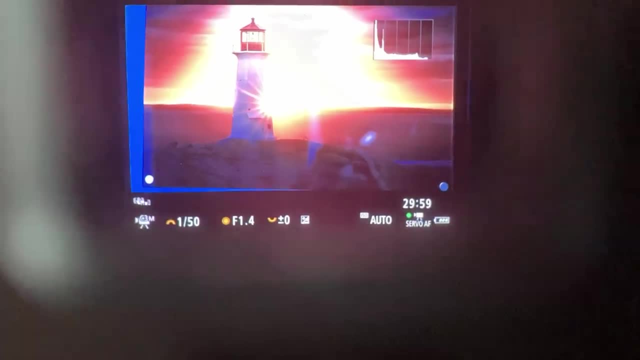 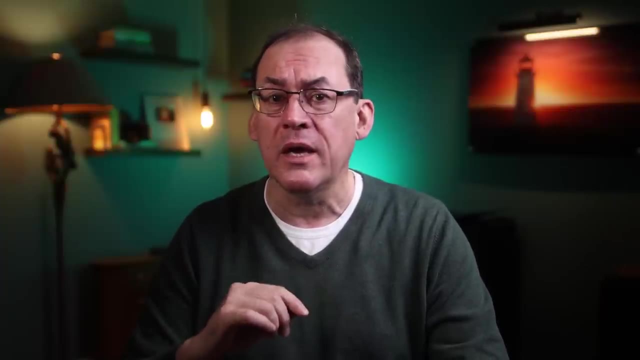 LCD showing you the photo You're about to take. The main benefit of this is that your camera will show you what your photo will look like, including how dark or how light the eventual photo will be, which DSLRs don't do. This is a great feature. 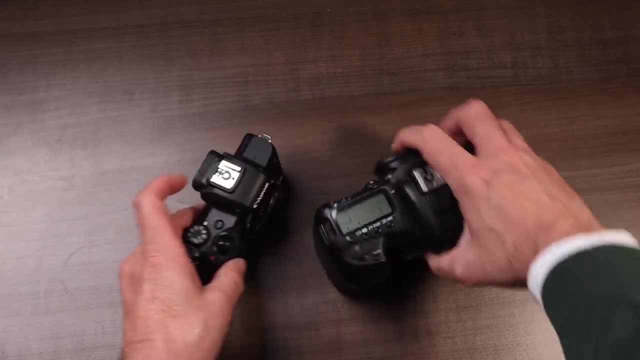 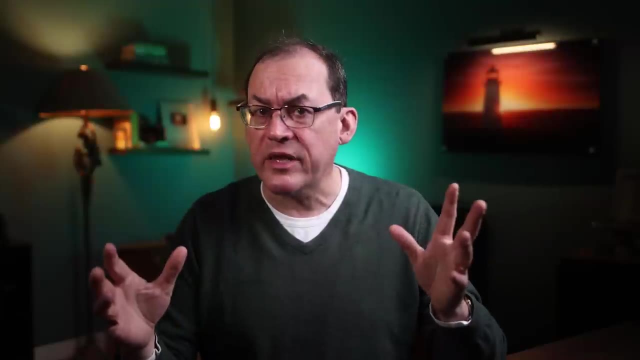 Mirrorless cameras can also be made smaller. If you compare these two cameras, you can see how small the mirrorless camera can be made, even if the sensor size is the same. Cameras are currently going through a technology transformation, where mirrorless cameras are. replacing DSLRs. It's likely that in a few years, DSLRs won't even be offered anymore, Because DSLRs have been around for a while. there are lots of lenses available, but very few new ones are being made. Even if there are fewer available now, that means that mirrorless cameras are the ones 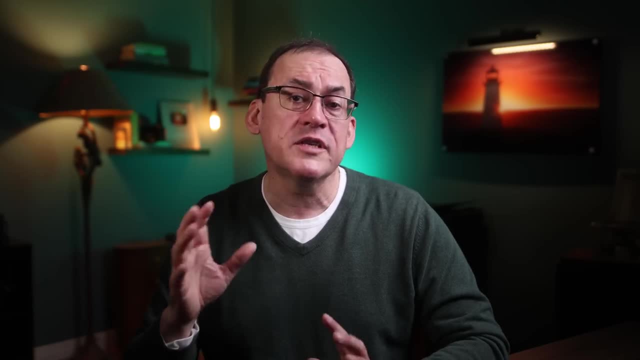 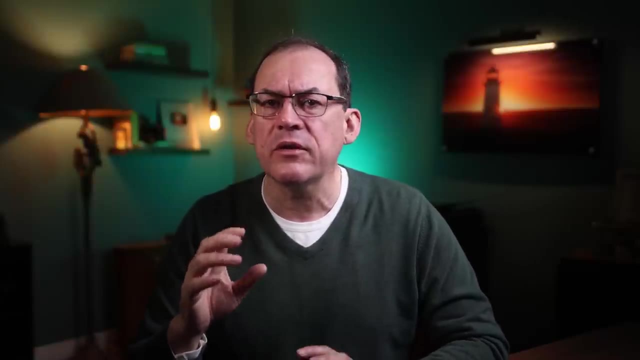 for which the new lenses and new innovations will be made. You can sometimes adapt DSLR lenses to mirrorless cameras, but not the other way around. Mirrorless cameras can also be shot silently, without a shutter noise- Great for a wedding ceremony or a music recital. 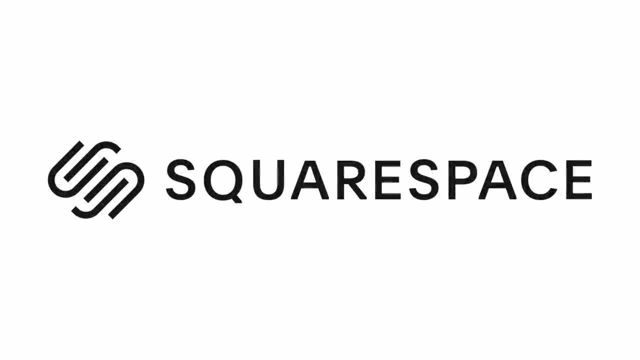 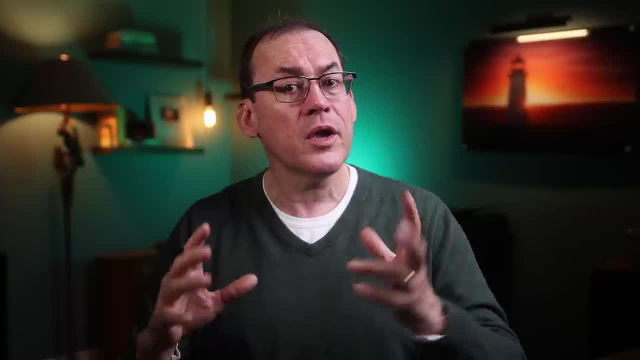 I'd like to thank the sponsor of this video: Squarespace. I created my own website using Squarespace and it was quick and easy. They have tons of templates to choose from or you can customize it as much as you'd like. 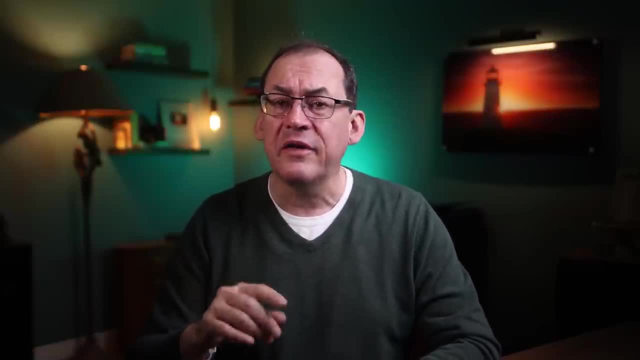 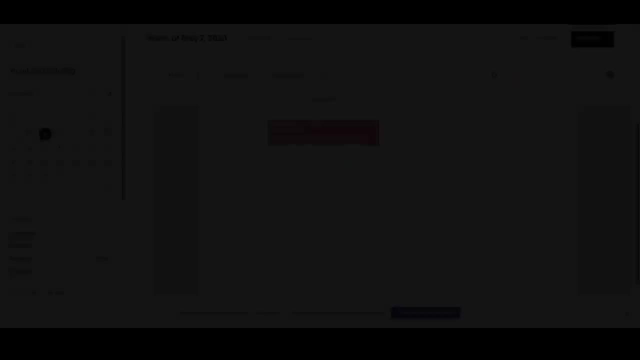 You can also use Squarespace extensions, which can connect your store to vetted third party tools like print on demand, to help you start selling products with no upfront cost. You can even add booking and scheduling for online classes. Clients can see when you're free and even reschedule if needed. 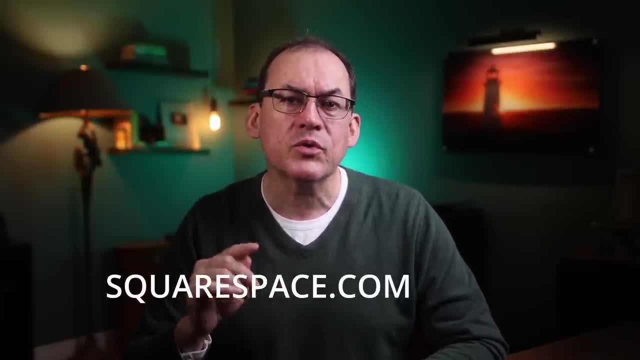 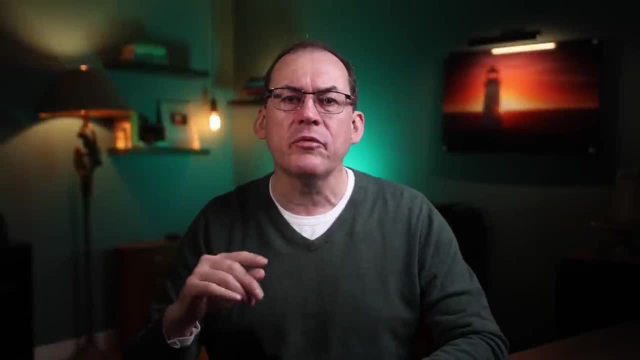 Head to squarespacecom for a free trial And when you're ready to launch, Go to squarespacecom- slash Simon to save 10% off your first purchase of a website or domain. While megapixels are often thrown at the front of marketing material about cameras, 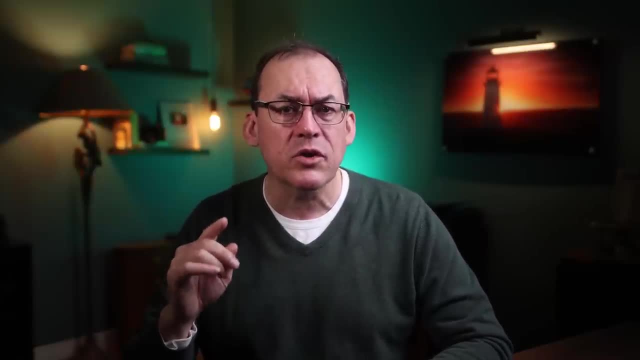 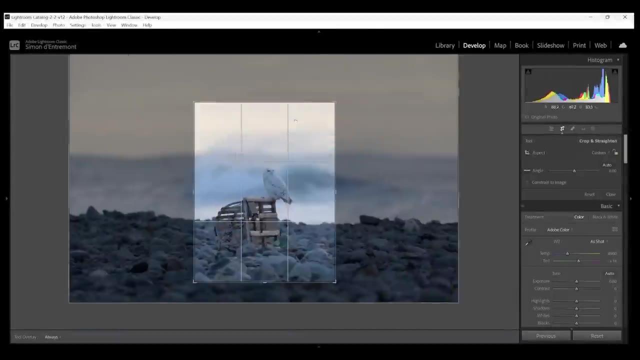 I'm going to go against the grain here and to suggest that you not make it your major criteria for buying a camera, unless you plan to crop your images. When cropping, the extra megapixels are really handy, as you can crop more deeply and still. 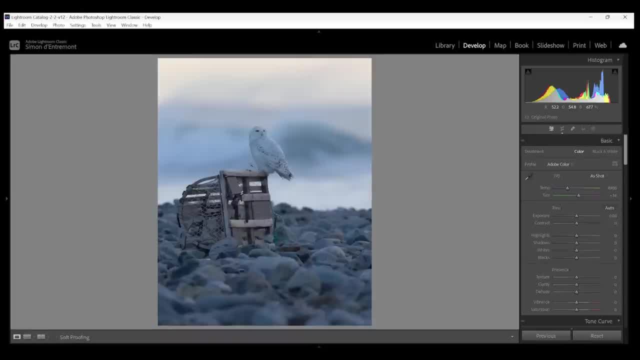 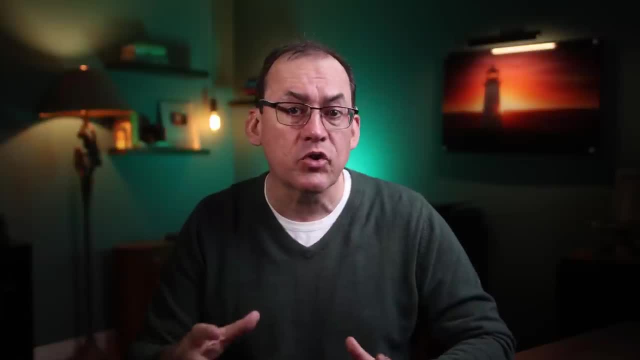 have leftover sharpness, So for wildlife and sports, for example, but if you're not cropping your images, most cameras today have enough megapixels To meet your needs of taking photos for your personal enjoyment or for Facebook or Instagram. Now, as for picking a brand, there's no right or wrong answer here. 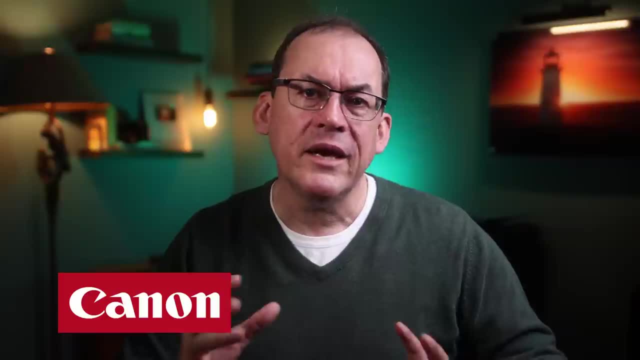 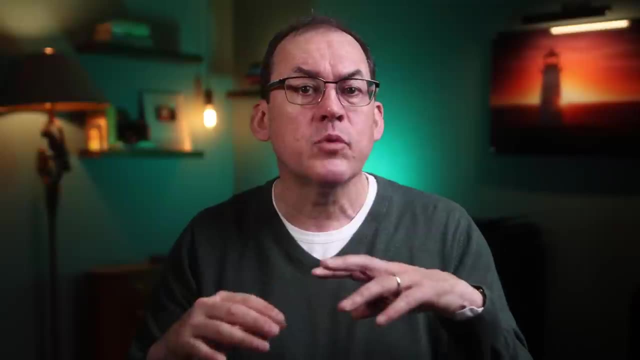 All the major manufacturers make cameras that can do a great job. Canon, Sony and Nikon have the largest market share and give you the advantage of having more lenses around in the used marketplace, as well as more online forums and users around to help you get advice. 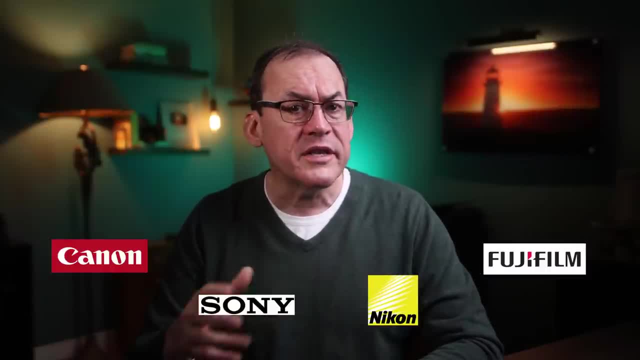 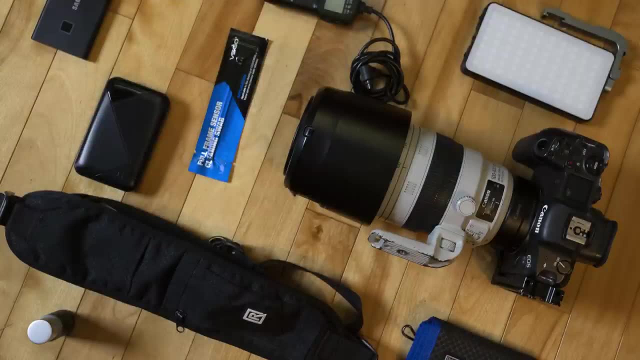 Larger brands also give you more options to grow into, with different sensor sizes and professional quality models. That's because you can't just buy a new lens and then just switch to a new one. It's a lot of further action. So I think that's the best way to get your future self to future proof yourself. That's because once you buy lenses, batteries and other accessories for one brand, switching later may be expensive. So my advice is: make sure your chosen brand can serve your needs if you want to grow into the hobby and start off with the brand that you want to stick with for the long term. 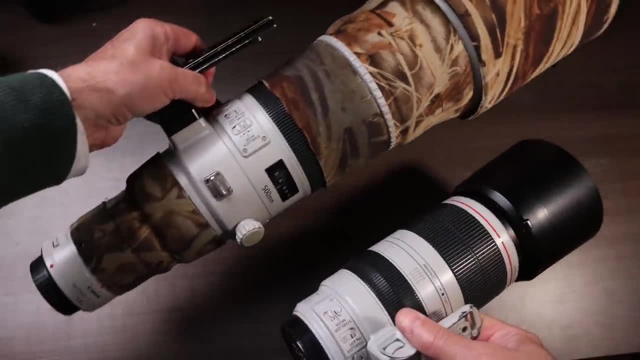 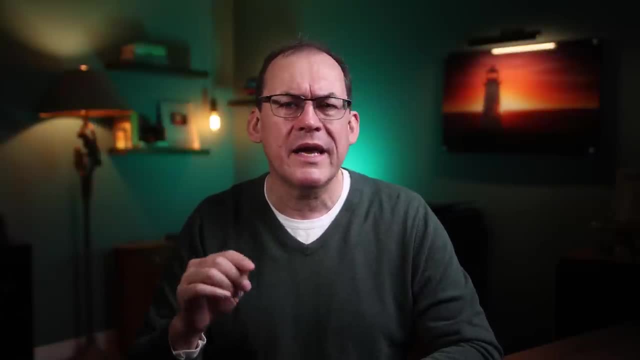 I started shooting Canon and still do, but not necessarily because they had the best entry level cameras. Sensor stabilization is a feature that's becoming more and more popular all the time, but it's often reserved for higher-end cameras. If you can happen to find in a more budget-friendly version, take it. 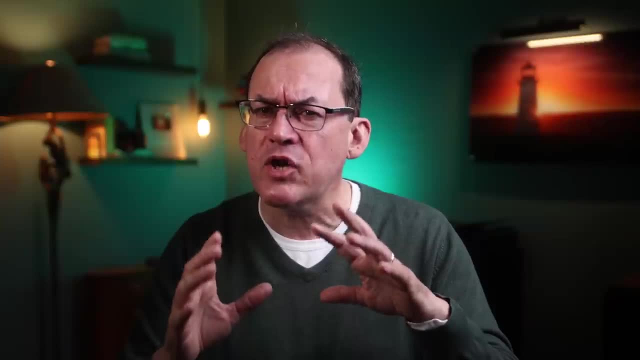 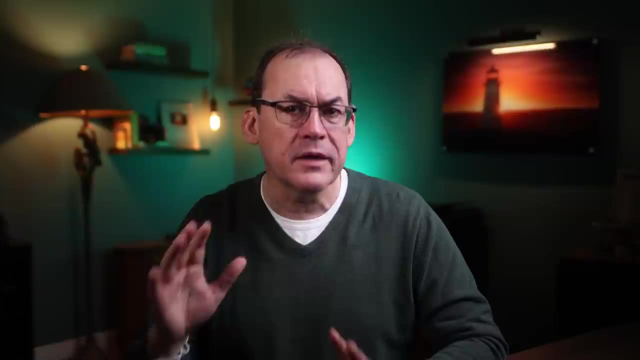 It makes it easier to get sharp photos in low light by allowing you to get sharp photos even if your shutter speed is really, really low. That being said, I've only been using it for less than two years, and before I had it, I could still get good photos. 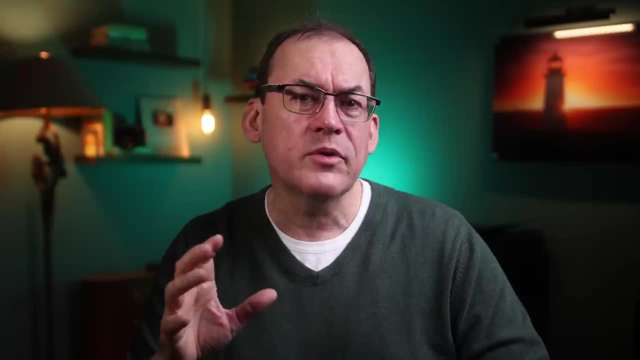 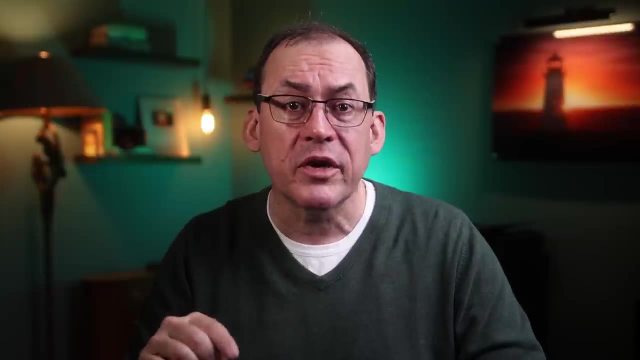 So don't pass up the right camera because it doesn't have it. Some cameras have digital image stabilization, which basically crops the image in a bit and moves it around to keep it still A decent feature, especially for keeping video footage smooth when walking around, for example. 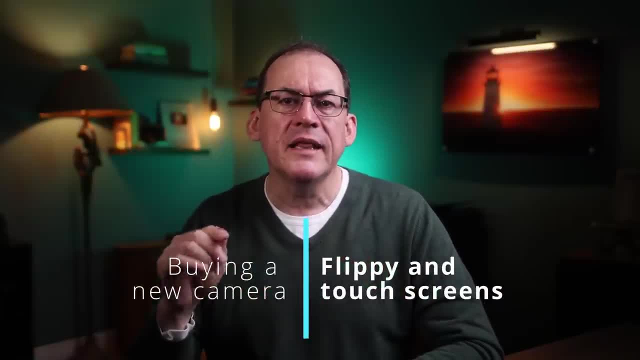 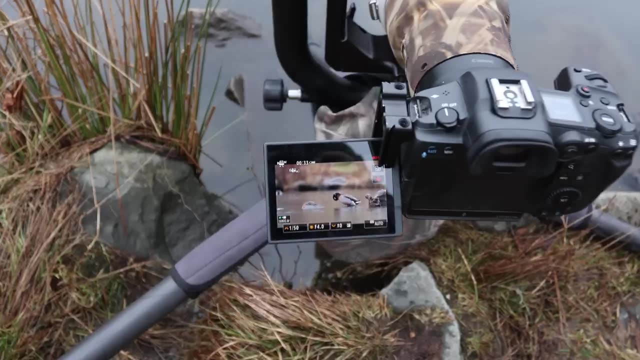 Articulating LCD screens are usually called flippy screens and they allow you to place the camera in awkward positions to get unique angles without doing contortions. I use this to get low angles for ducks because I like the look it gives my photos. 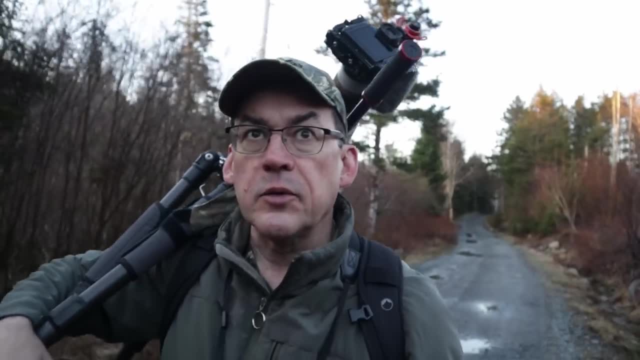 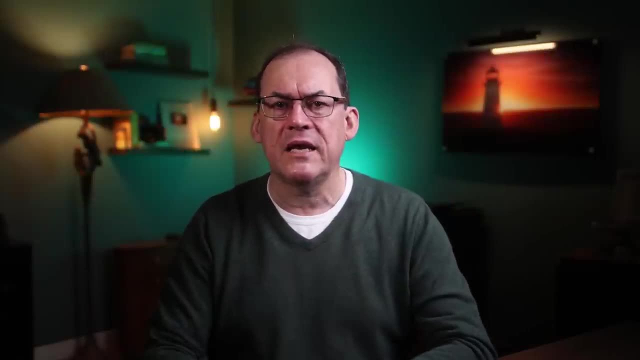 You can also place the camera higher to take pics or see yourself for selfies and vlogging. Some don't flip all the way around, though, and only lean upwards or downwards- Not mandatory, but really, really handy feature. Some back LCDs also have touchscreen capability. 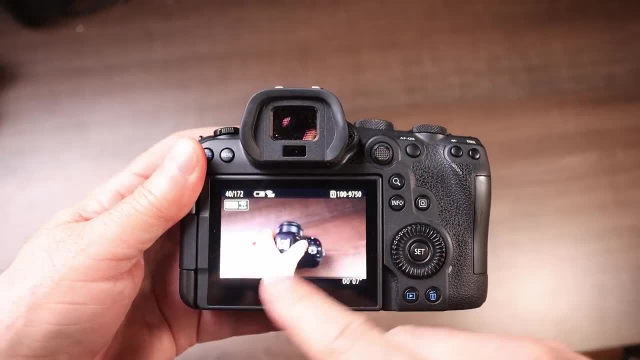 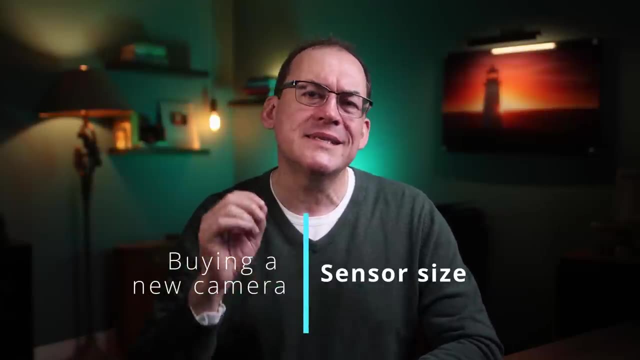 for menus settings, setting focus points and scrolling through photos. These are great. You can easily do without, but they add a great convenience. One of the big decisions you'll need to make is sensor size. Sensors start off with phone sensors that are very, very small. 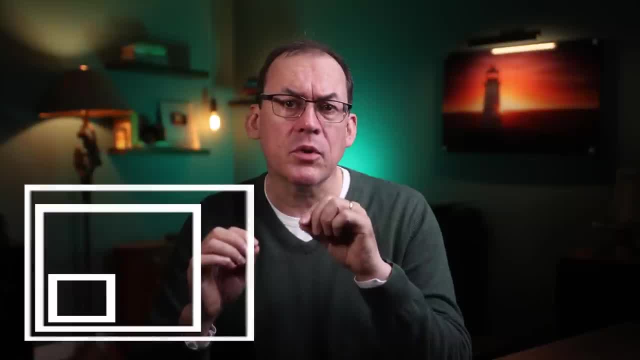 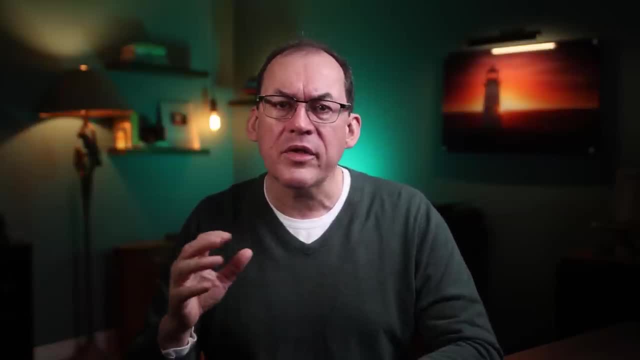 then micro, four-thirds or a bit bigger crop sensors, also called APS-C, a bit bigger still and finally full frame. Generally, the larger sensors cost more and are often paired with other features, which makes them even more expensive. Full-frame cameras start at $1,000,. 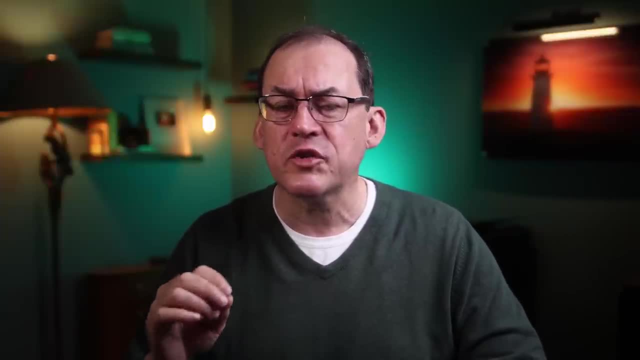 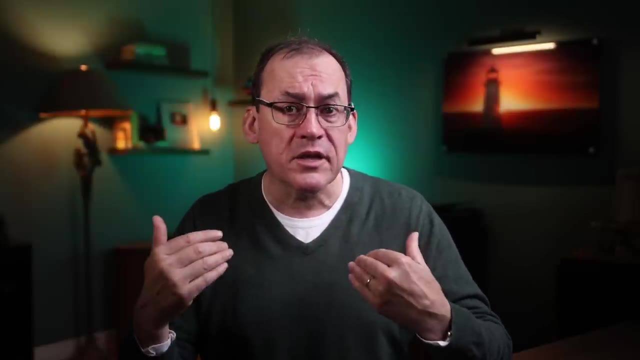 and many models over $2,000, so make sure you need those features before you get one. Most people's first cameras will have smaller sensors, like APS-C, and there's nothing wrong with that. That's where I started and where many people will start. 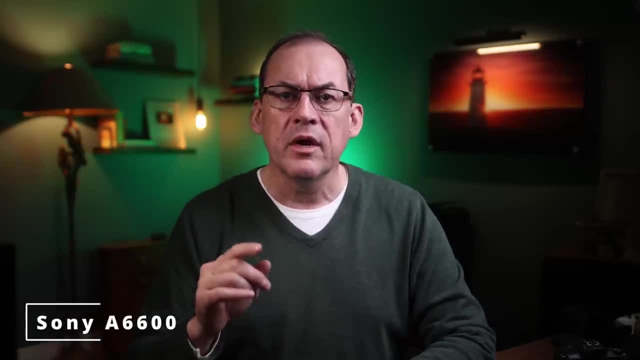 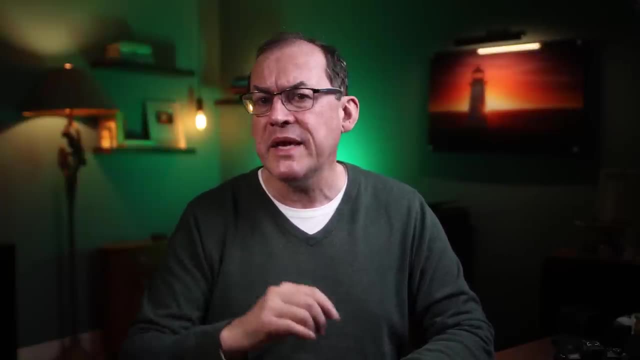 In APS-C size sensors. the Sony a6600,, Fuji X-T4,, Nikon Z50, and Canon M6 Mark II are all optional. They're awesome and have more features than basic models. That being said, manufacturers are noticing that people with decent phone cameras 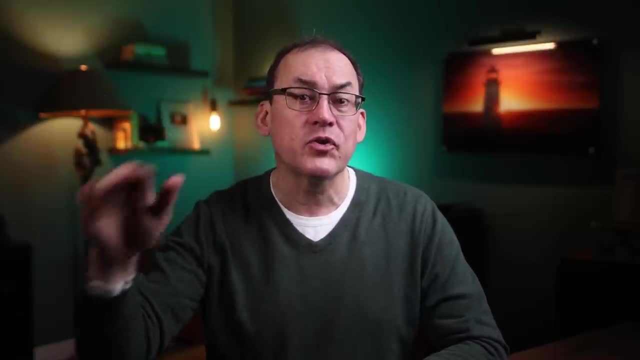 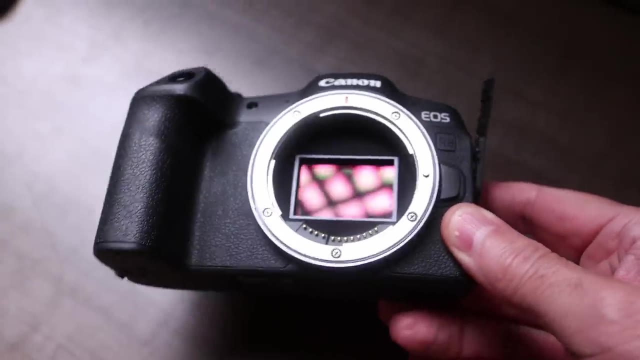 who want to upgrade may want to jump right over a crop sensor right into full frame. so lower-priced full-frame cameras are coming out all the time. There's never been a better time to get a full-frame camera as your first serious camera, if your budget can handle it. 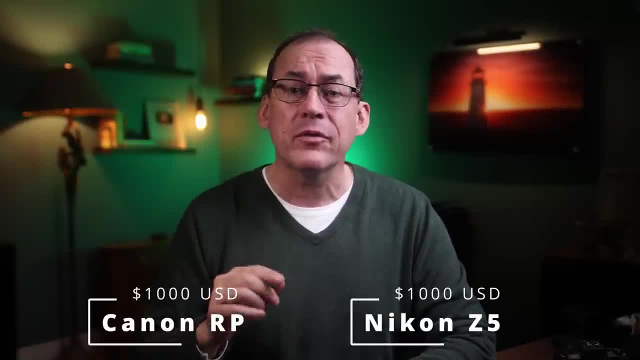 Canon's RP and Nikon Z5 can be had for around $1,000 US for a great start to full-frame. Canon's new RP and Nikon Z5 can be had for around $1,000 US for a great start to full-frame. 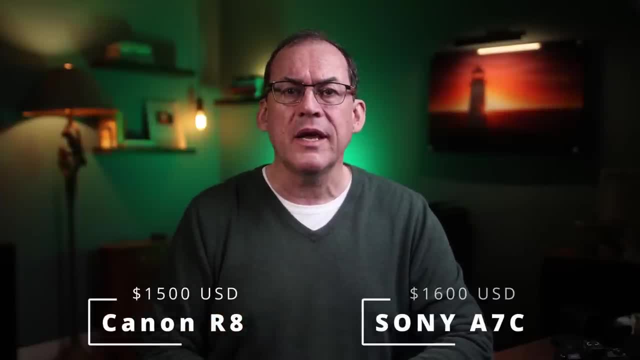 Canon's new RP and Nikon Z5 can be had for around $1,000 US for a great start to full-frame. The Sony R8 is a wonderful new addition at a low price point and Sony's a7C is a great way to enter the Sony system without breaking the bank. 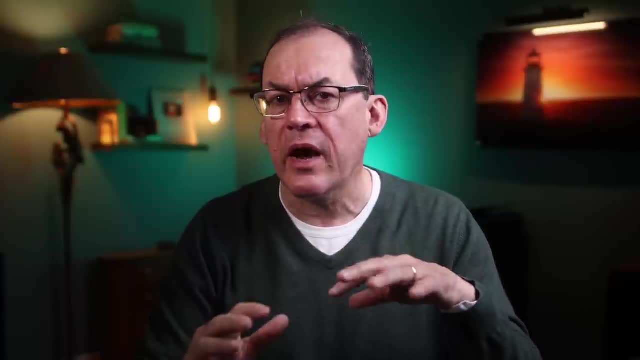 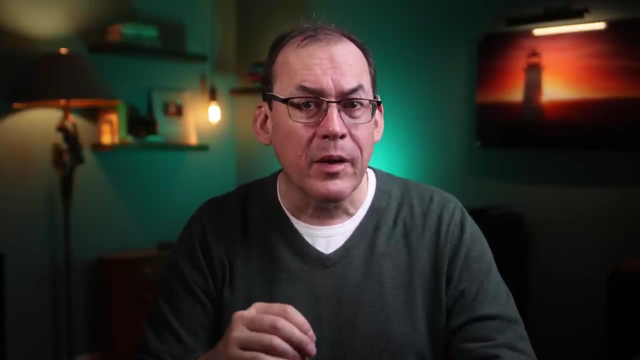 Choosing a sensor size is best made by looking at what you will photograph. Larger sensors are better in low light, so a full frame would be a better choice for night photography, dark environments like indoors, music venues, dark theaters or wedding receptions. 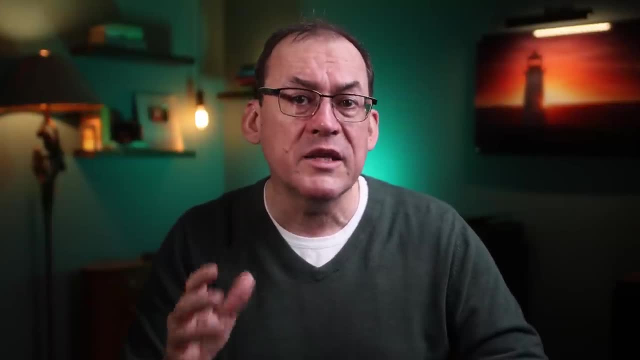 Smaller sensors may struggle in these environments. On the other hand, smaller sensors have a different performance. On the other hand, smaller sensors have a different performance advantages too, While they capture a smaller section of the image circle created by the lens. 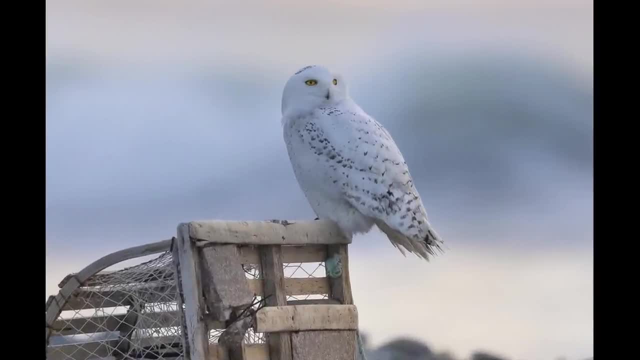 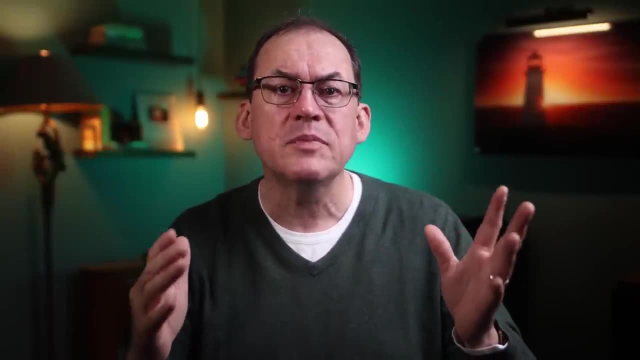 when you enlarge it to fill the screen, it gives you an effective magnification. So smaller sensors like Micro Four Thirds and APS-C give you more reach for sports and wildlife. Full frames can be great for wildlife and that's what I use, but you need to buy very. 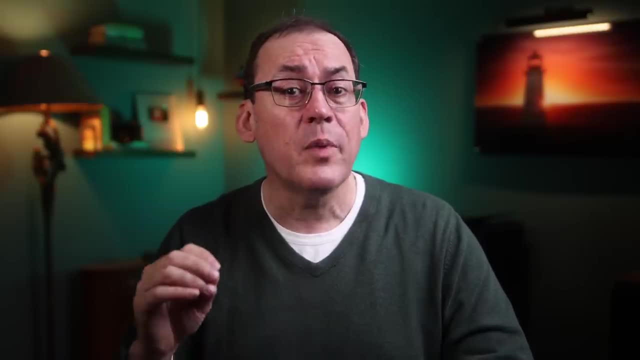 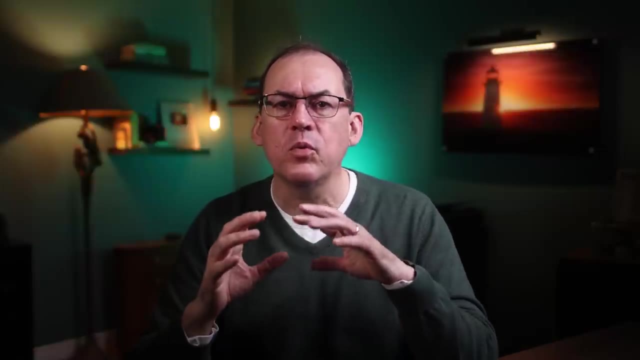 very expensive lenses to get the reach that you need. If I was buying my first camera for sports and wildlife, I'd get an APS-C or Micro Four Thirds. Micro Four Thirds are a favorite of people who want small form factor cameras, light and easy to carry around. Olympus and Panasonic are 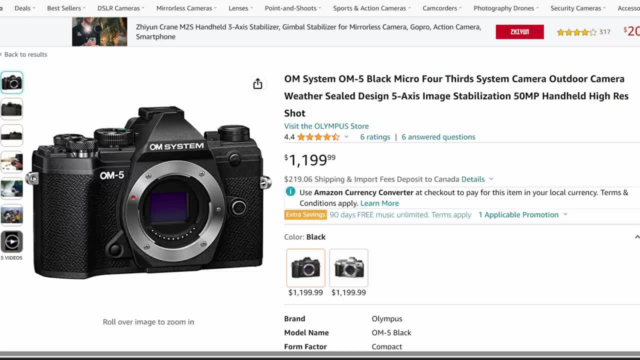 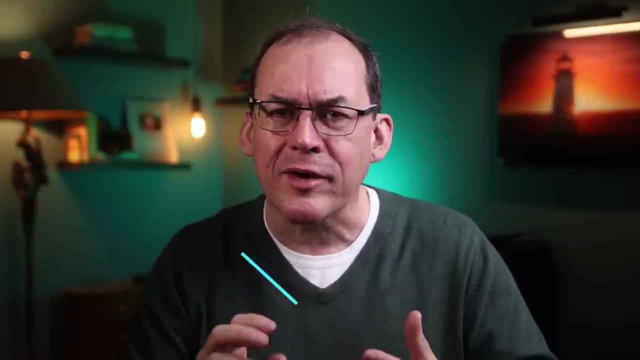 brands that are chosen for these. The Olympus OM5 is a favorite in this category. Another consideration is if you're going to be shooting video which is growing in popularity, either TikTok or your kids playing soccer. Some cameras have very good video features and are sometimes 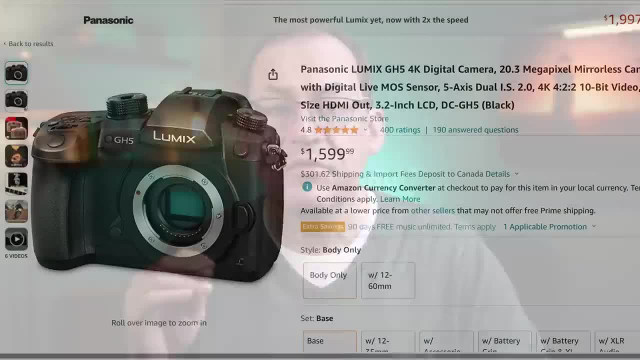 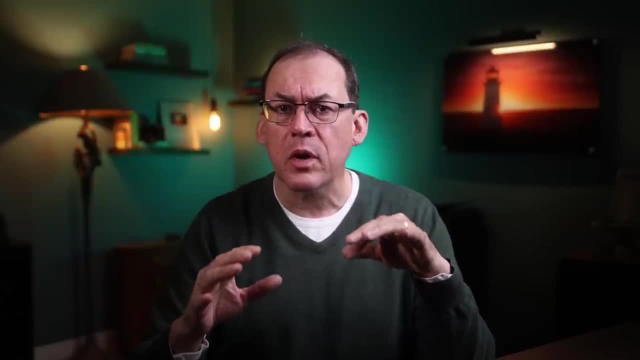 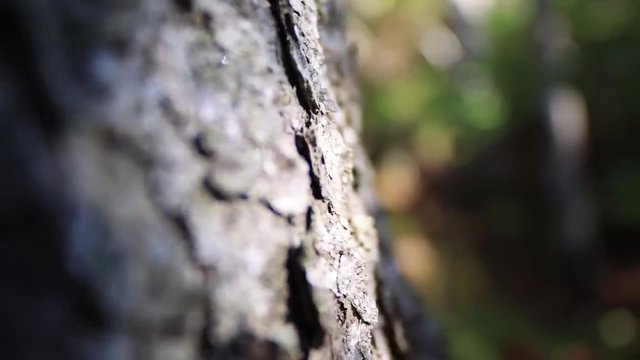 called hybrid cameras because they do both photography and video Very well. 4K, which is not needed in all genres, is becoming a new standard, though, and will future-proof your video work, as people are watching sources like YouTube and so on, more on big TVs, more often. 4K slow motion at 60 frames per second is a great feature for social. 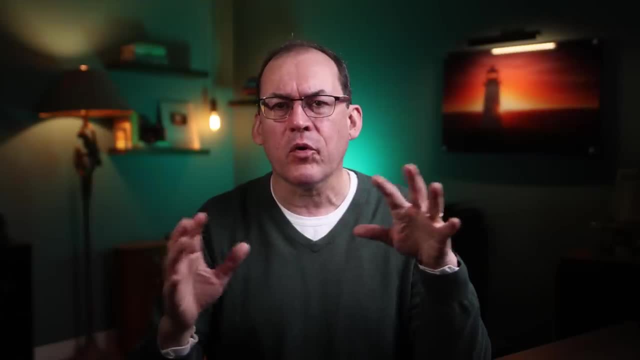 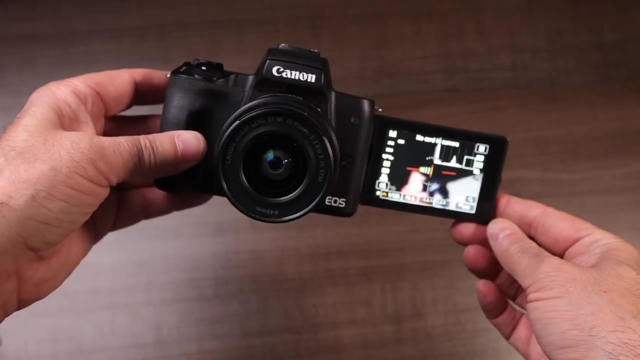 media work and artistic forms of video, but less important for recording of family outings. If you're going to use it for things like vlogging, make sure you get one with a flippy screen to see yourself and a mic jack, because the stock audio on cameras isn't very good. 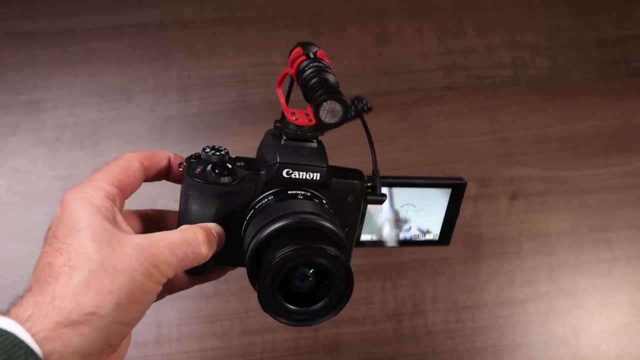 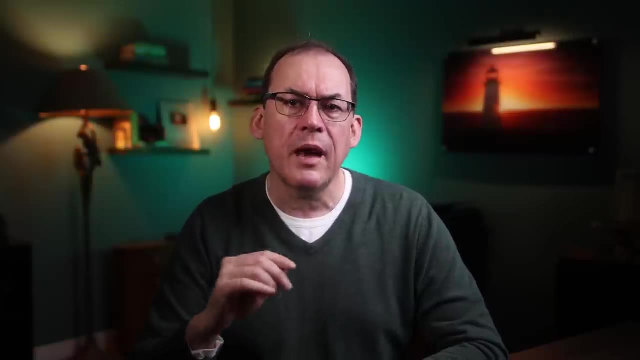 At a smart price: A small shotgun microphone like this one, which you can get for under 50 bucks and you're good to go For vlogging. you also want eye detect so the camera can focus on your face. Mirrorless cameras are a better choice over DSLRs for this, due to their eye detection features. 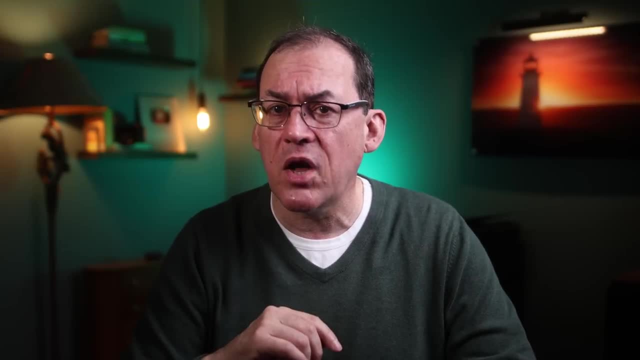 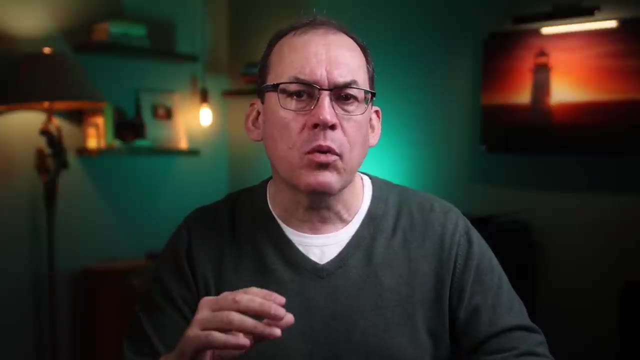 This little Canon M50 Mark II is an example of a great little vlogging camera. The Sony ZV-1 and ZV-E10 are two other great choices. If you're shooting action or wildlife, you have two other very important criteria to 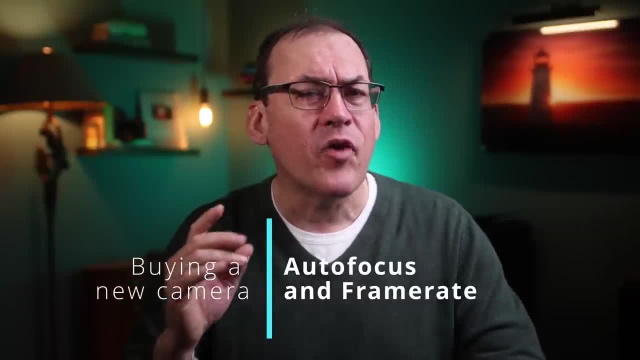 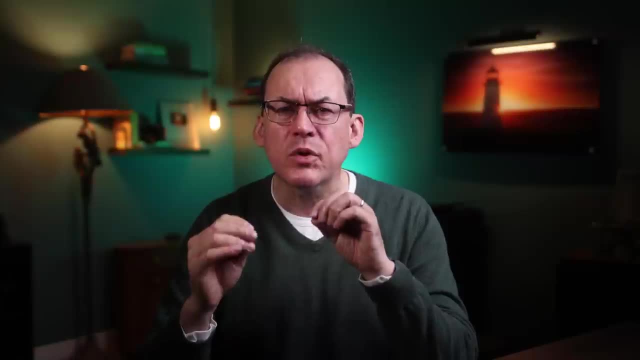 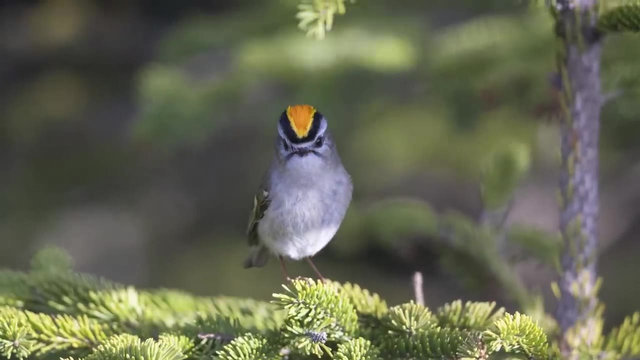 consider. While autofocus is important in all photography, for action, sports and wildlife, it's the most important criteria. Also, having the ability to shoot many frames per second allows you to capture those peak moments and the best odds of great photos. Having five to seven frames per second or more is a decent amount, and ten frames per 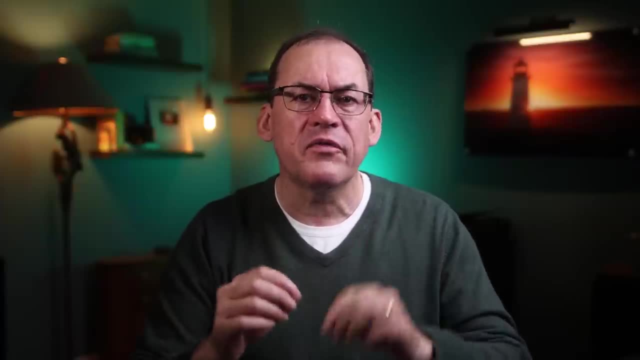 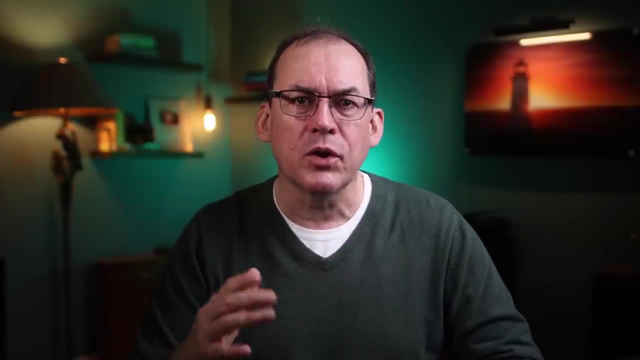 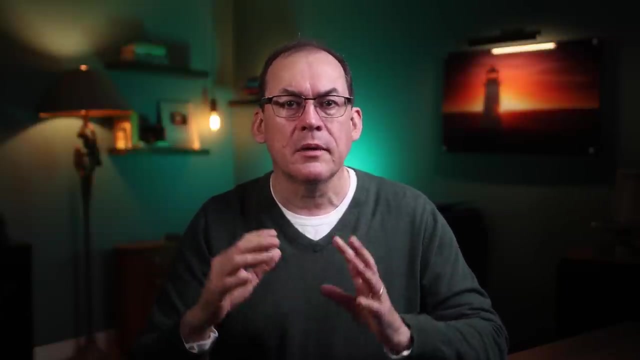 second, you're golden. Evaluating focus ability is very difficult off the spec sheets. While it's beneficial to have more autofocus points than less, for example, the ability of the focus point to lock onto your target isn't easy to do. Checking reviews by users who photograph the same subjects you do like: animals, motorsports. 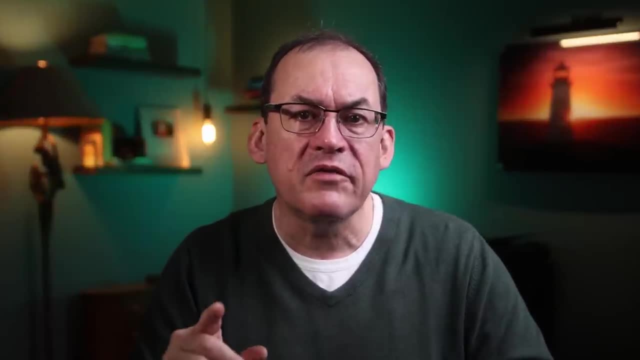 or swimmers in a pool is a great idea. Nikon's D500 and D7500,, for example, are great DSLRs for wildlife and action like birds in flight, and have a better autofocus system at this point than the mirrorless beginner. 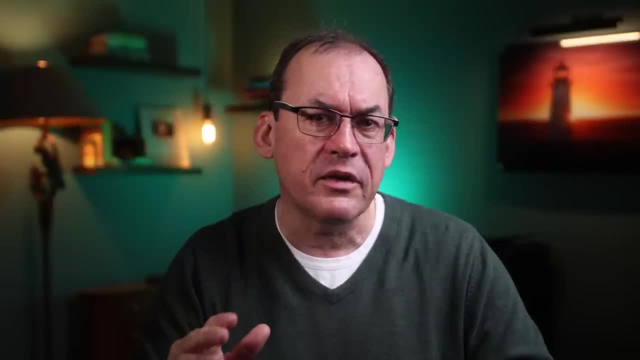 or intermediate offerings of the same brand, like the Z50,. if you're shooting challenging subjects like birds in flight, Canon's mirrorless R50,, R10, and R7 are great cameras. Canon's mirrorless R50,, R10, and R7 are great cameras. Canon's mirrorless R50,, R10, and R7 are great cameras. Canon's mirrorless R50,, R10, and R7 are great APS-C mirrorless action cameras. Canon's mirrorless R50,, R10, and R7 are great APS-C mirrorless action cameras. 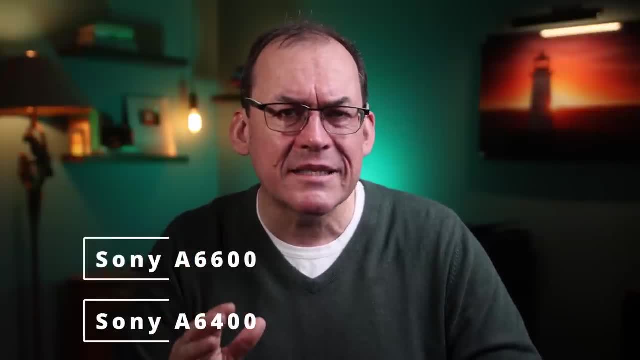 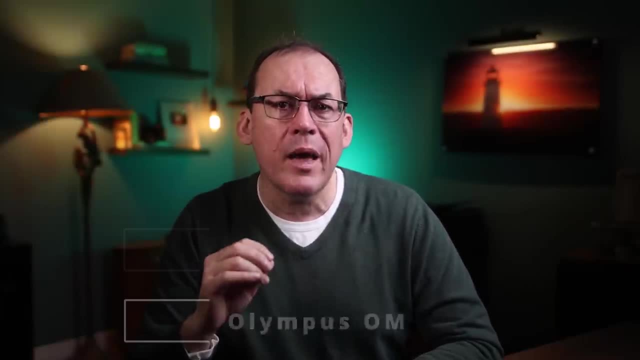 Canon's mirrorless R50,, R10, and R7 are great APS-C mirrorless action cameras. Also Sony's A6400 and A6600, Fuji's X-T30 and X-T4, these are all great choices In the micro four-thirds arena. Olympus OM and E-M series are great choices for action. 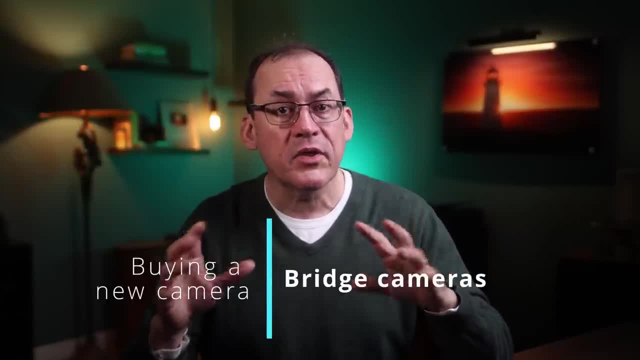 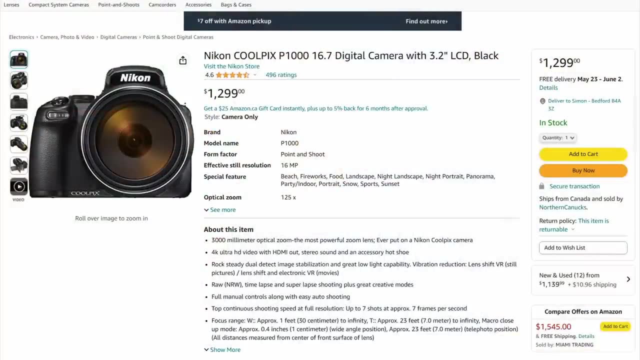 as well as the Panasonic G9.. If you only want one camera that can shoot really wide but still have tons of reach at the same time, without switching lenses, then you want what's called a bridge camera: bridging the gap between point and shoot and interchangeable lens camera. 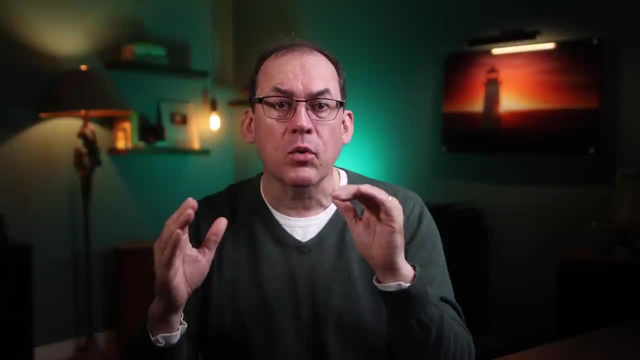 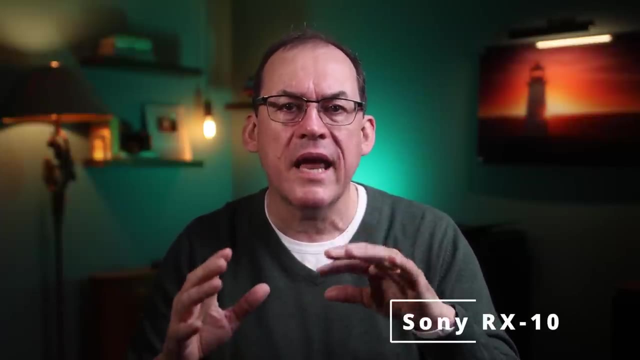 bridging the gap between point and shoot and interchangeable lens camera. These have a fixed lens that goes really wide to really deep. The Nikon P1000,, Canon Powershot SX70, and Sony RX10 are great and popular choices, Even if they cost a bit more than other cameras on your list. remember that you don't need. 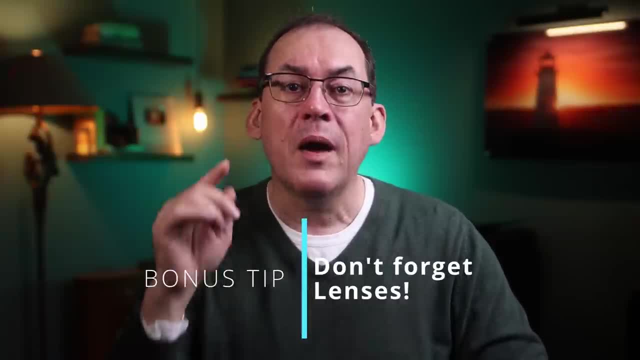 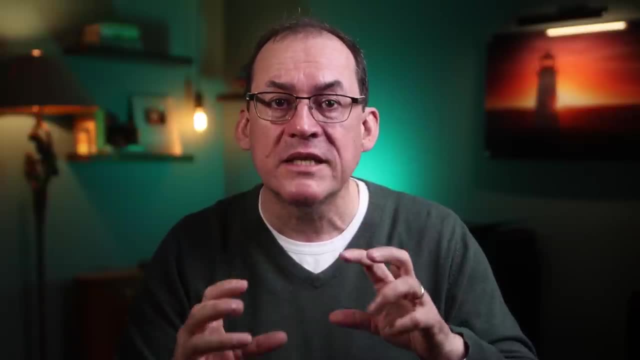 to leave room for lenses. But speaking of lenses, my most important piece of advice is: don't spend all your time and budget worrying about a camera and forget about the lenses. They are just as important as the camera And in some genres, like wildlife, I'd say more important. 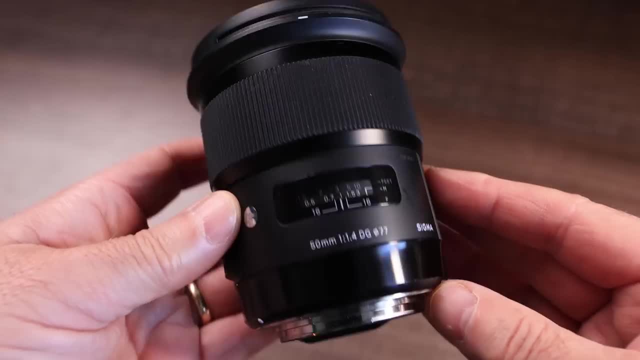 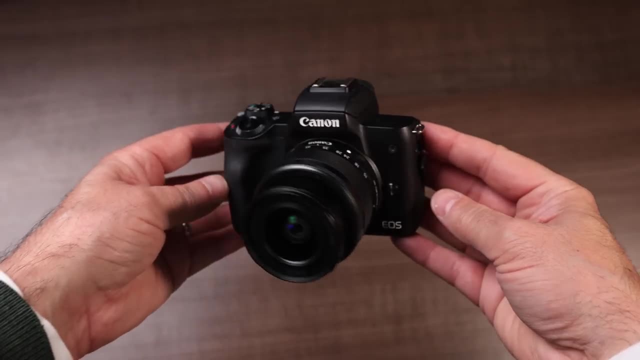 Before you buy a camera, make sure that the lenses you need are affordable and available. Your camera may come with what's called a kit lens. To keep the price of the camera down, this lens usually isn't the best quality, although on some higher end cameras they may pair the body with a decent lens. 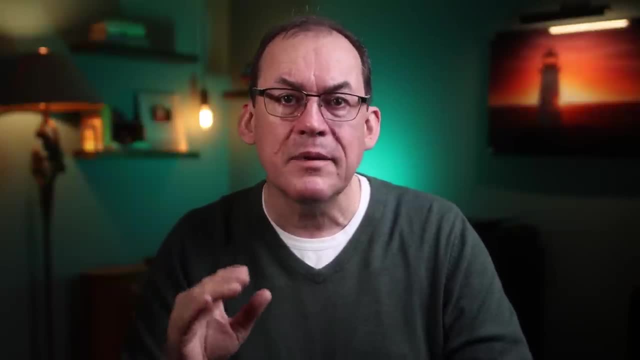 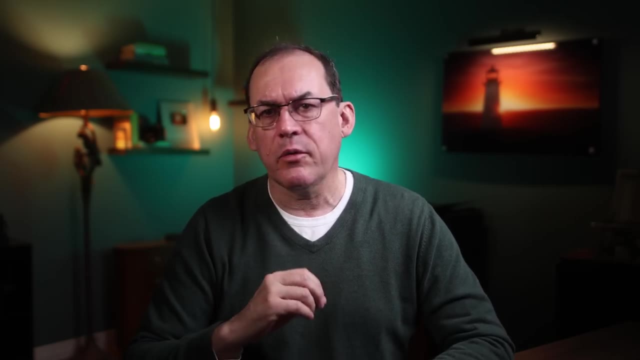 A lens upgrade or buying the camera body with no lens and buying a great lens for it is a really, really good choice, Strongly recommended. It's a great place to start with your first camera. That's because they're flexible and adaptable and avoid needing to bring along various lenses. 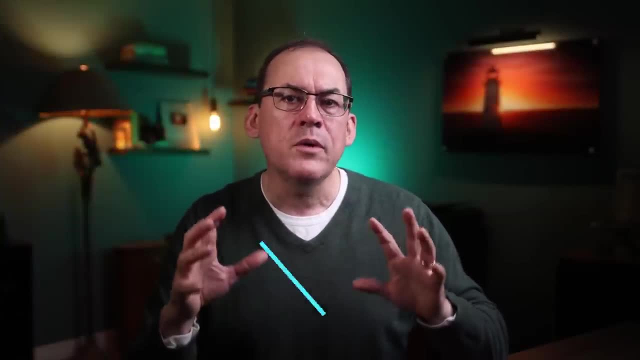 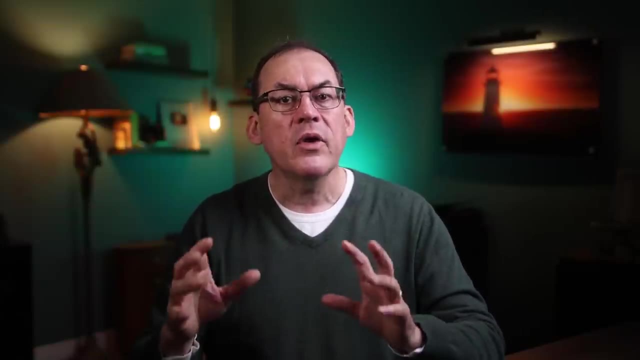 of fixed focal lengths called prime lenses. I wouldn't buy an expensive one until you know what focal length you use the most. See what experience tells you first. If you have a 24-105mm zoom and all your pictures end up being shot at 24mm, then that's your. favorite focal length, Then a 24mm prime might be in your future And that would be the time to get one. One exception may be for buying your first prime lens is that most manufacturers make an inexpensive but decent quality 50mm f1.8, often called the nifty 50, a couple hundred. 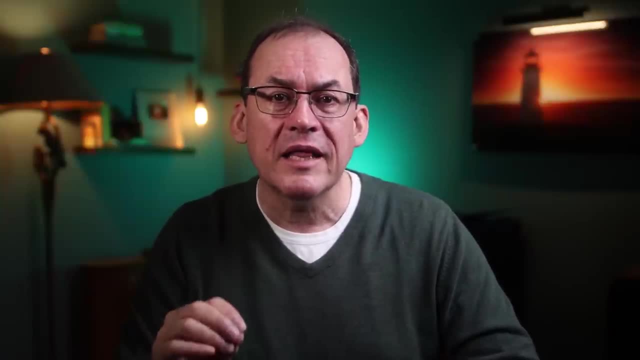 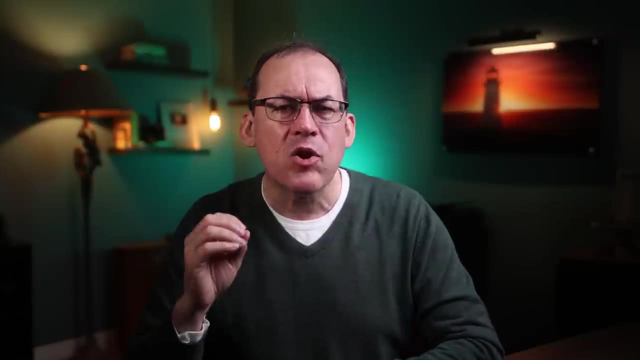 bucks and easy to find. used, That's often a great lens and often used focal length and lets in a good amount of light for better image quality. Worth getting. So when it comes to lenses, a great lens will turn a decent camera into a great one by capturing. 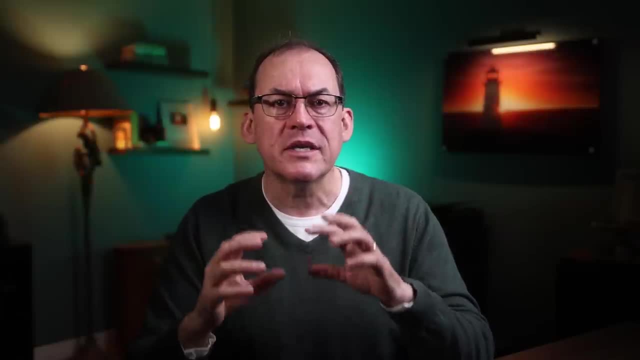 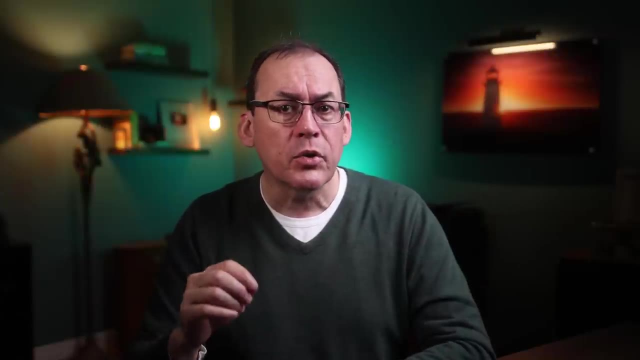 more light for better image quality and delivering sharper images, Especially if you're looking for a better image quality If you shoot in dark environments like music concerts, indoors or at sunrise and sunset, Don't splurge on a good camera and put a crappy lens on it.